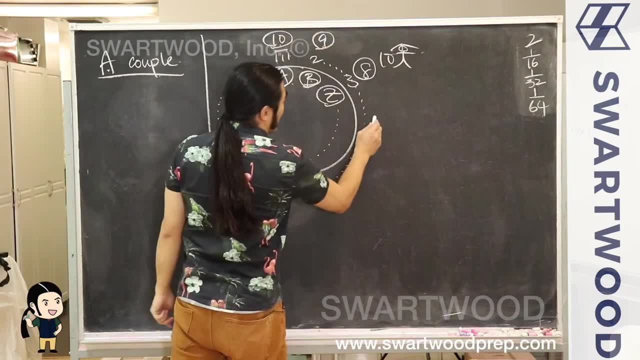 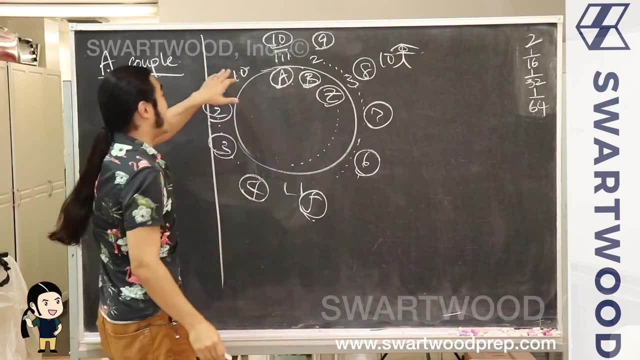 all the way around And you can see. that's kind of interesting. It's going to be ten, nine, eight all the way down. So times seven times six times, five times, four times, three times two, And then, when we get to seat number ten, there'll. 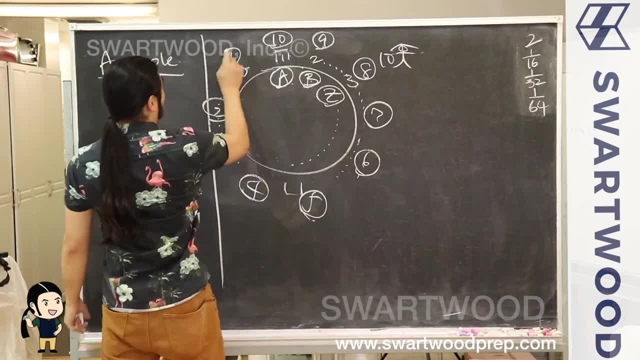 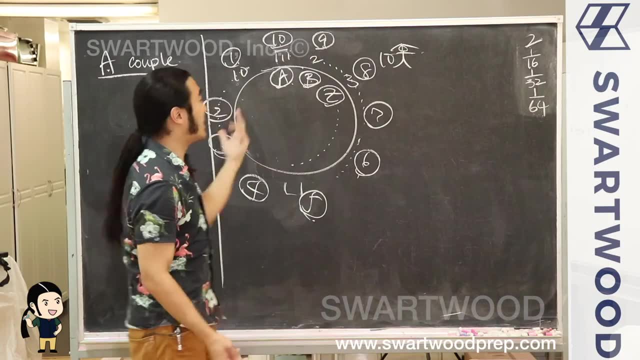 only be one seat left and one person left, so there's only one choice over here. Okay, Remember our rule of thumb: In the middle of making choices, we multiply. So you have ten options here, then nine here, then eight here. That looks like it's going to be ten. 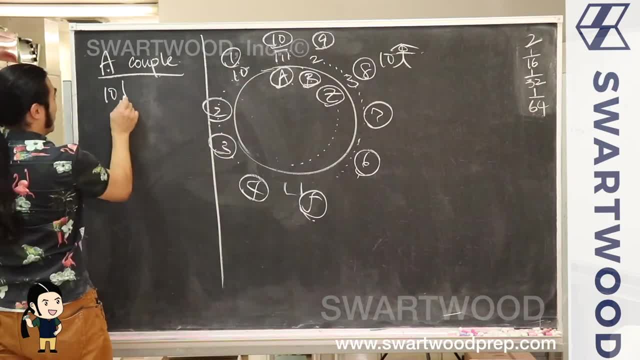 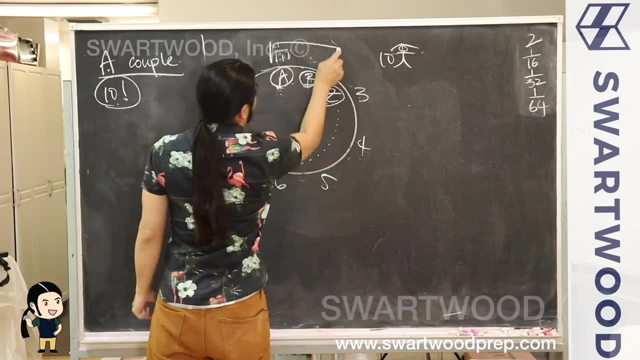 times nine, times eight, all the way on down. so it's going to be ten factorial. Okay, All right, That's the total number of possible seatings. we can get What about the couple right? So let's see. So we can put the couple down, maybe here. 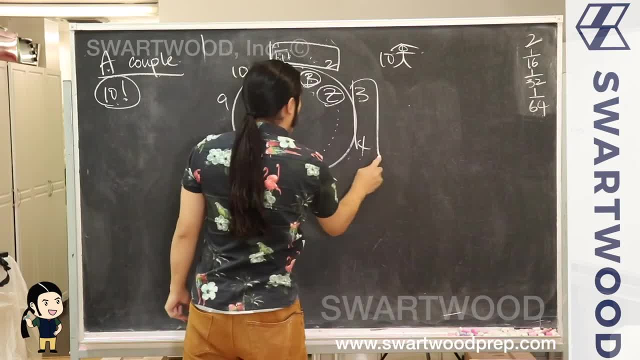 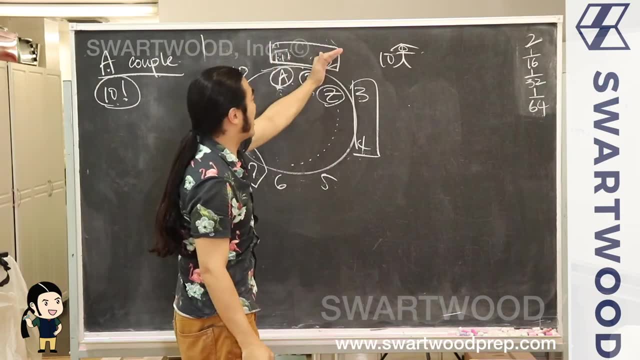 right in order for them to sit together, Or maybe we can put them down, say here or here, something like that. Does everybody agree? So we'll do it this way. Let's imagine there's a left side and a right side, okay, or a side that's more counterclockwise. So 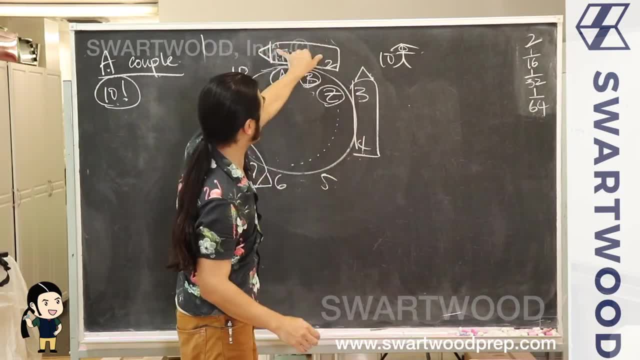 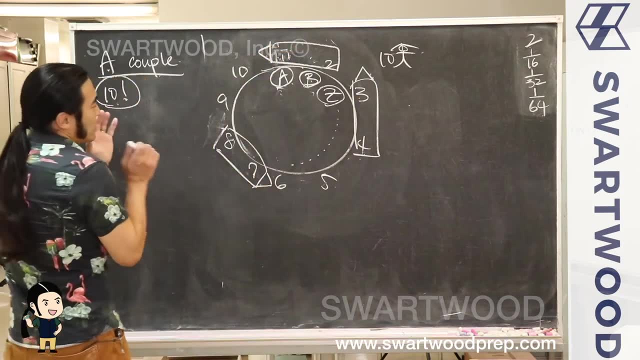 here on this side, we'll distinguish it like this: So we're going to put that block of two down and we're going to look at the side that's more counterclockwise. So it'll be like this, And then over here it'll be on this side. Okay, All right. So to know where. 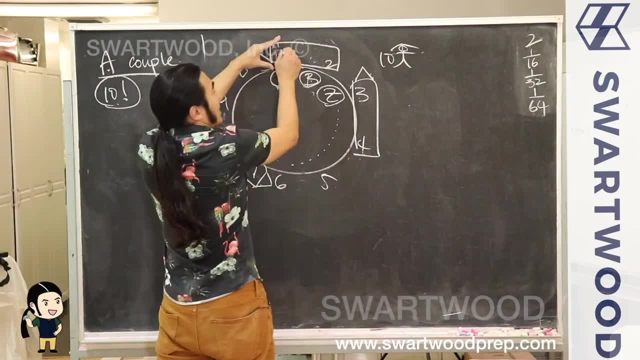 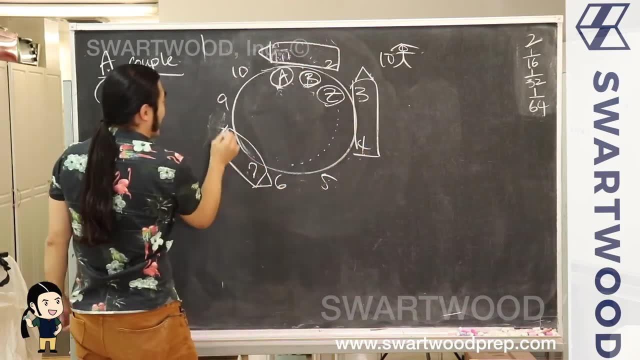 that block sits, we pick the counterclockwise, So we're going to look at the side that's more counterclockwise, right? How many places can I place this side, the counterclockwise side? We can do one. Well, apparently one, two, three, four, five, six, seven, eight. 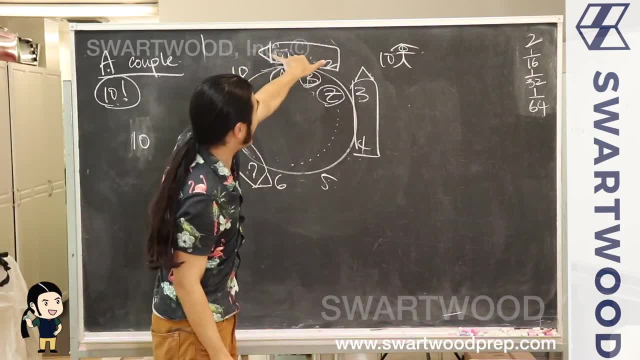 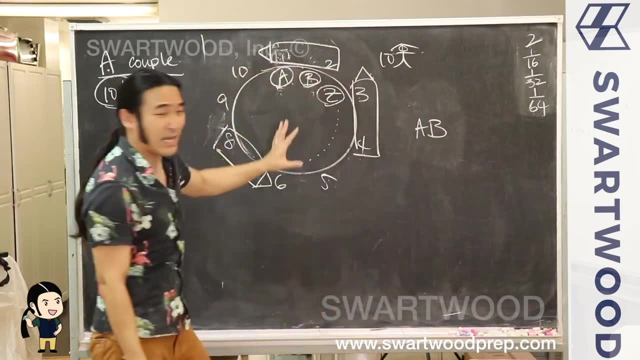 nine, ten, Okay, No big deal. But once we place that down right, we still don't know what that block looks like, because you have the couple. Let's say the couple is say A and B, Okay, So if you want to sit A and B down together in this setup here in this, 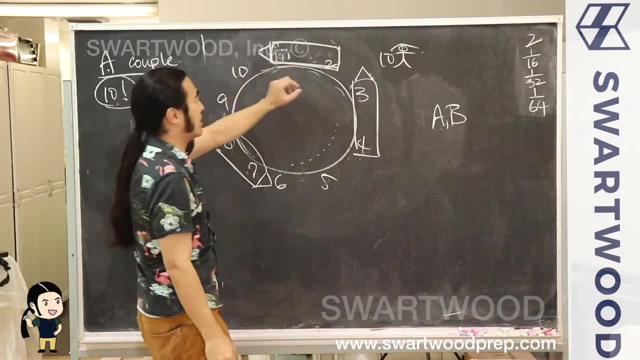 particular one. I'm going to say left and right because it's kind of easier to talk about than counterclockwise versus clockwise, But you know what I mean. So if you look over here, right, we don't know if A is on the left. 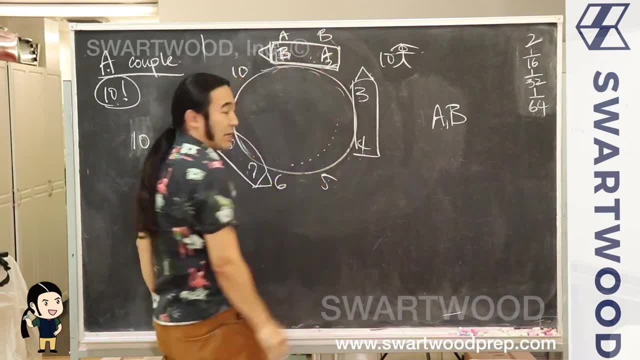 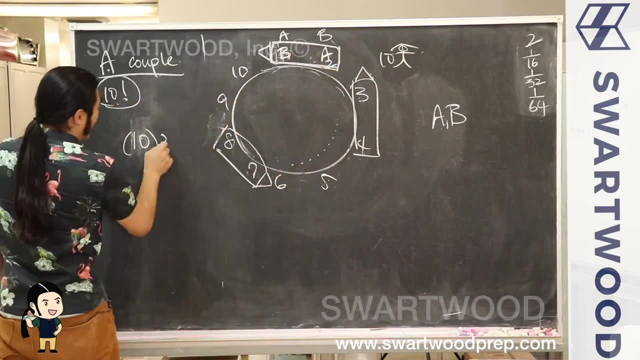 And B is on the right, Or B is on the left and A is on the right. So for every placement of that block we have two possibilities, right? So in truth, what we really get is ten times two. Okay, So now we do our basic probability thing. The number of ways Remember. 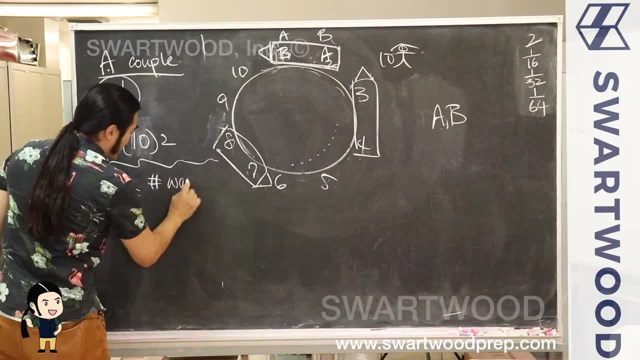 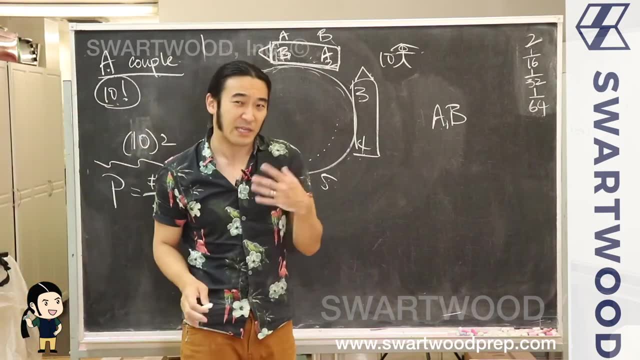 the classic way of thinking: probability is the number of ways of getting what you want over a total number. Okay, And in here, if we think of all these possibilities being equally likely, this will work. Okay. So what are the total number of possibilities? 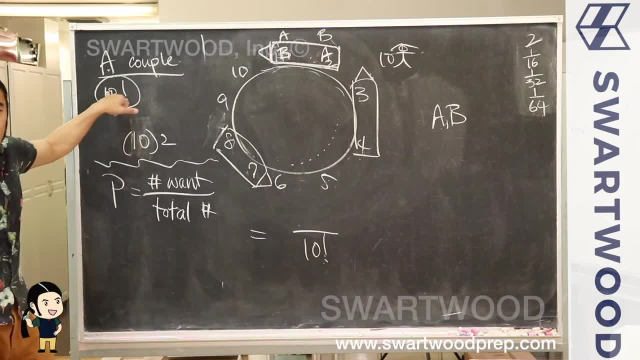 Whether it's a number of possibilities. whether it's a number of possibilities, whether it's ten factorial possible setups. Okay, We computed that, How many of them give us what we want? Well, apparently, ten times two are twenty. So we get twenty up top here. Okay, But is 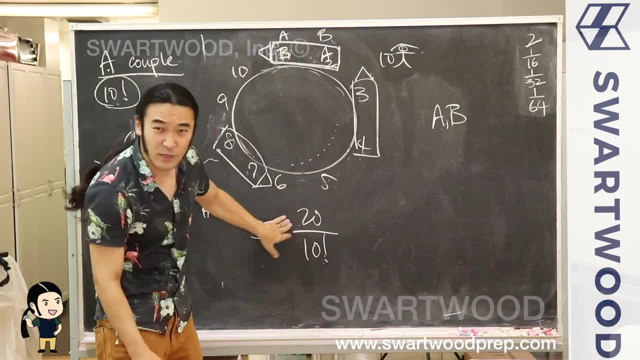 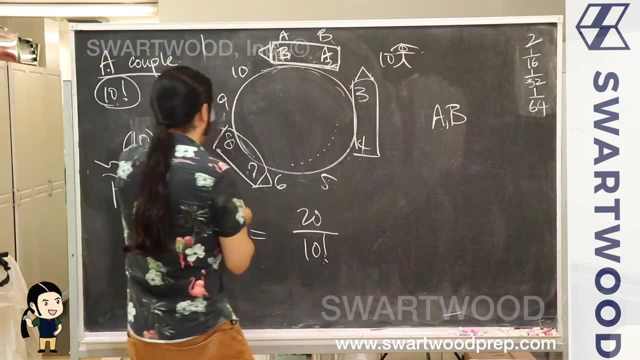 that completely right. Not quite, because what we've actually done here this is close, but we've placed the couple and we know where they sit, but we don't know where everyone else sits, So what we really need to do is finish out the rest of this. Okay, So imagine, 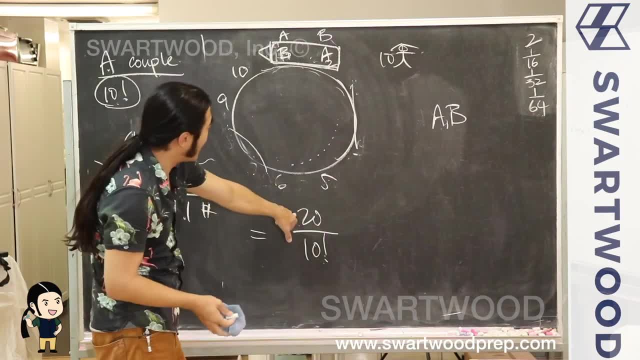 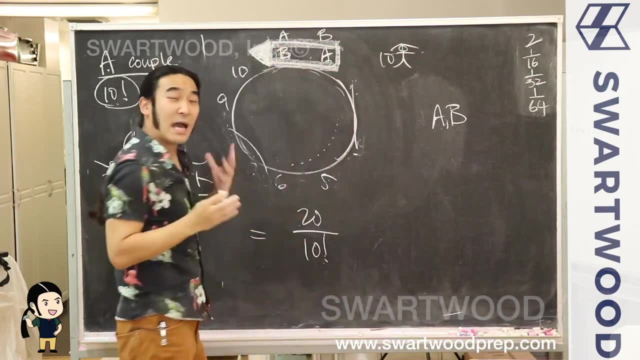 in our scenario again. So for these twenty we're counting. So for every setup in here, we know where the couple sits, right, But we don't know where everyone else sits. So once we place the couple down somewhere, Okay. So now we know where the block sits. 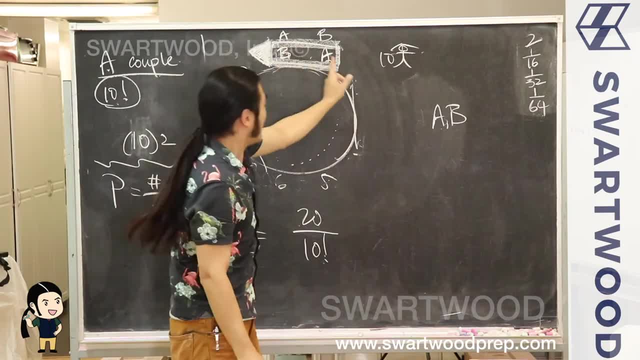 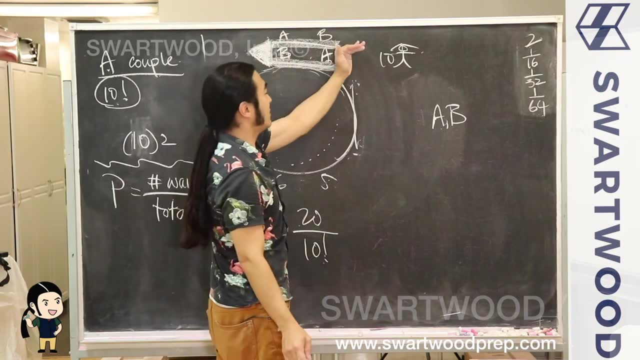 We know where these guys sit relative to one another at the block right, But in this setup here we don't know where everyone else sits. So if you look at the seat over here, so let's call this the head and this the tail. If you look over here, the seat, that's next. 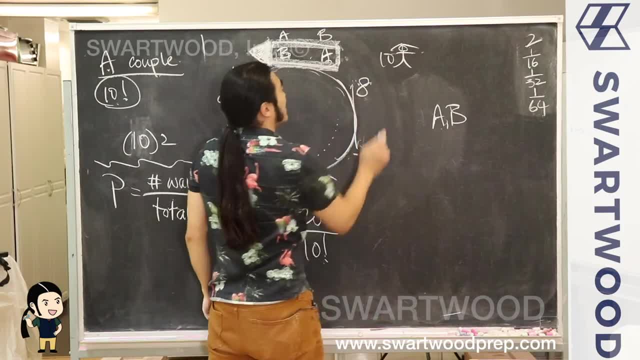 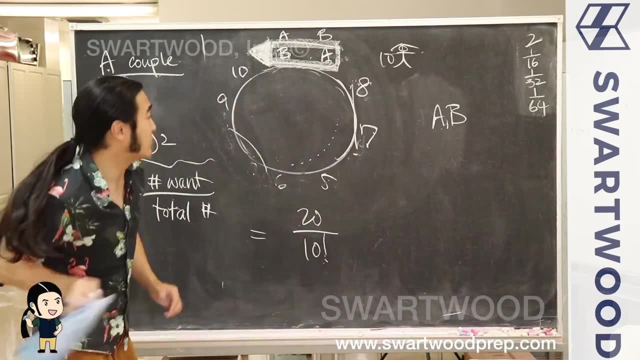 to the tail. well, two people are used up, So that gives you eight possibilities left for who's sitting over here right And just like before. that means for the next seat, how many possibilities are left? Seven, And we keep working. In fact, we work our way. 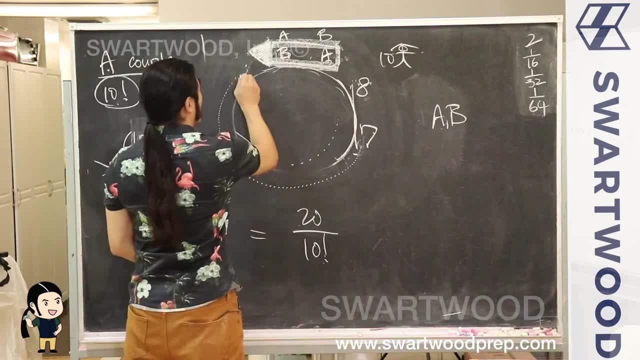 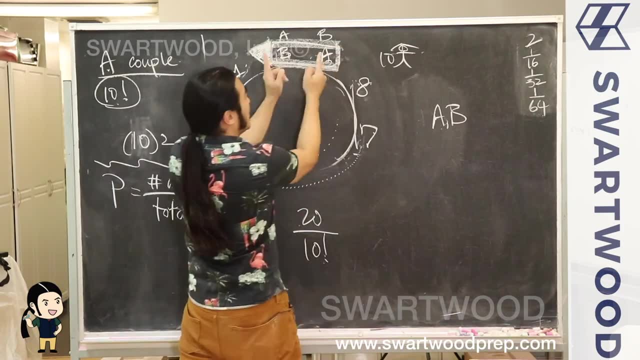 all the way down Back to one. Does everybody agree? So the truth of the matter is it's ten choices where we put the head of the block Once we place that block down. there are two choices where we put the two people in the block right. Once that's done, we still have to make, apparently. 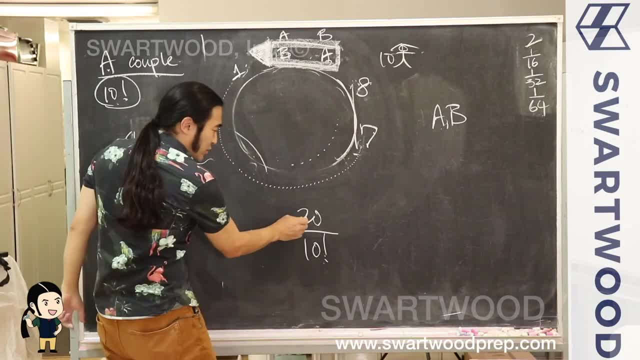 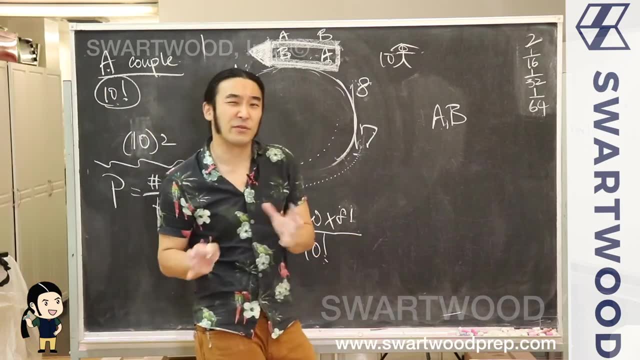 eight factorial choices for where everyone else sits. So the right answer is really twenty times eight factorial. Okay, Now I think we're good. So when we first work through this, we figured out we know where the couple sits and we know who's sitting at the head. 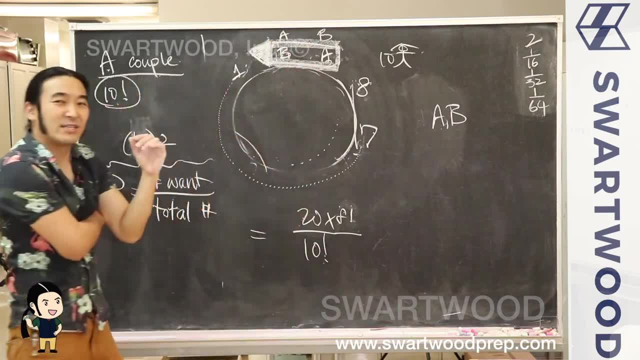 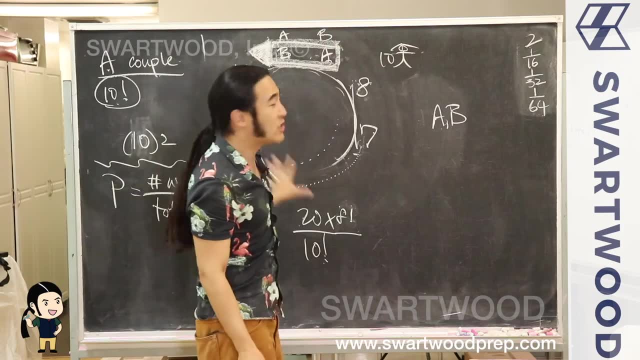 of that block right And we don't know where everyone else sits. And the question isn't figure out where the couple is. The question is figure out all the possible arrangements where the couple sits next to one another. So you have to have the entire arrangement done to know what. 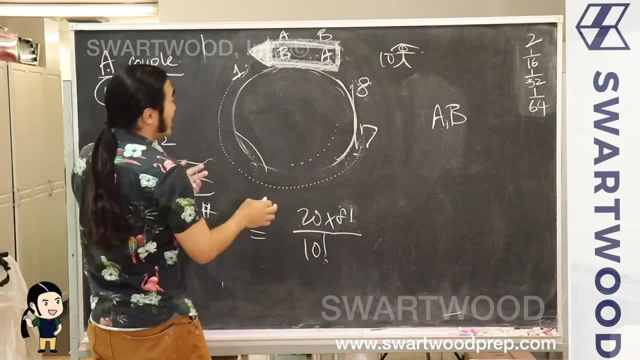 everything looks like Okay. So, with that in mind, we know we're good, because what we really need is just a complete arrangement, right, All right. So what are the arrangements we're looking at? We're looking at ten possible places where you put the head of the block. 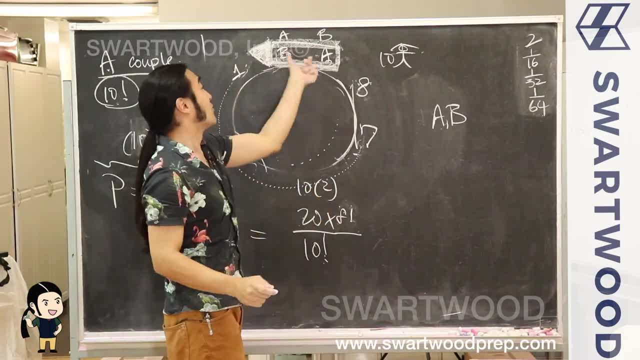 Okay, And for each one of those setups there are two places where you can move around the people inside the block. Okay, But then after that there's still what Eight factorial possibilities for where everyone else sits. Okay, So we're good, So we're good, So we're.